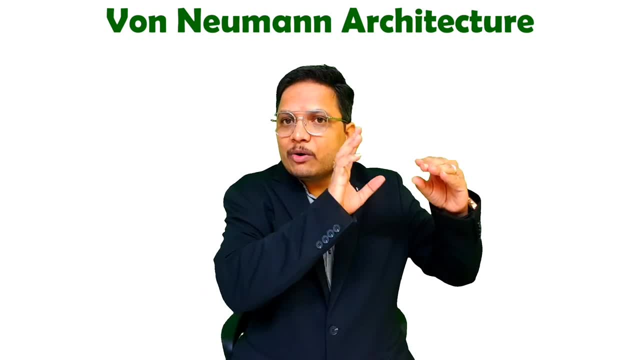 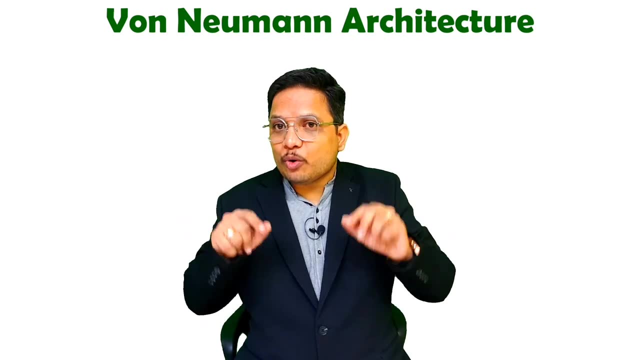 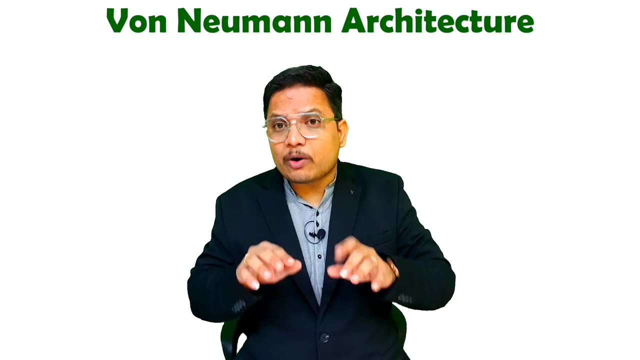 So what will happen? when you double click on PPT, you will be opening this data inside a program, and that program is Microsoft PowerPoint. When you open this, at that time you can read the program as well as here. you can modify the data as well. 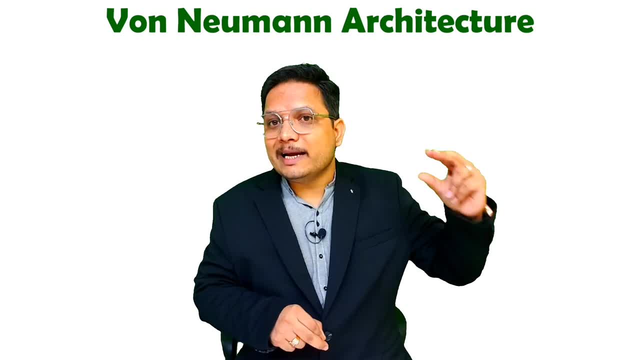 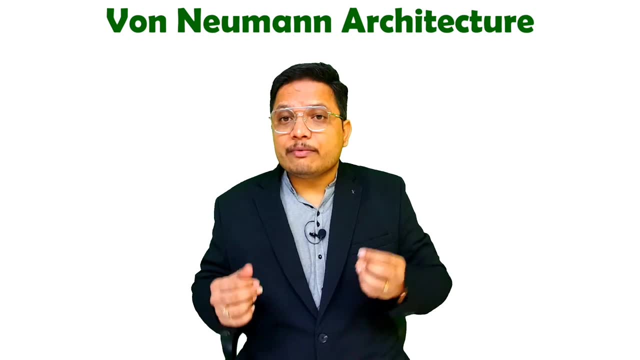 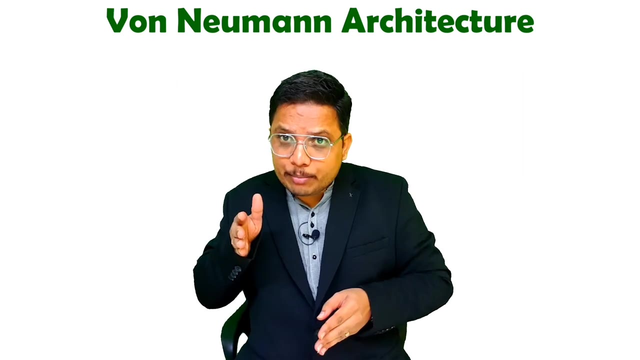 So whenever you edit the PPT, what will happen? That data will change. with video and with audio, We don't change data, but there are some data which may need to changed. So here, CPU that will be executing programs. Along with that, it will be accessing data. 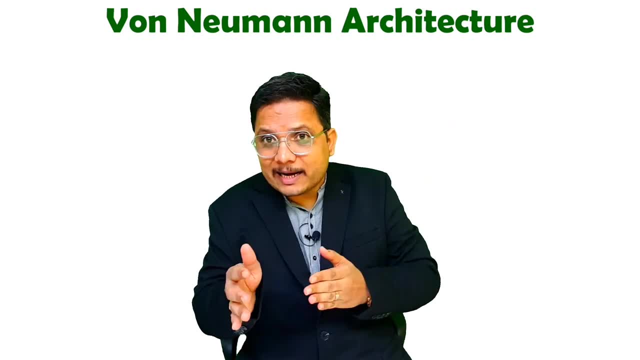 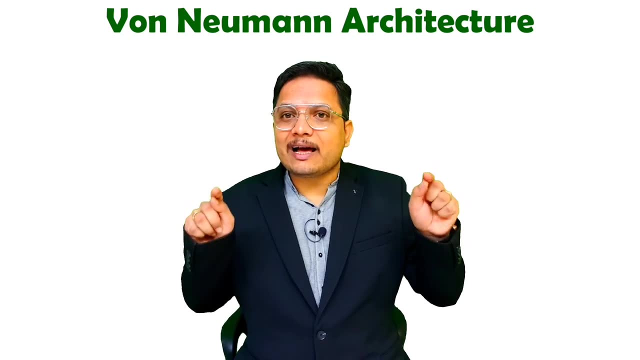 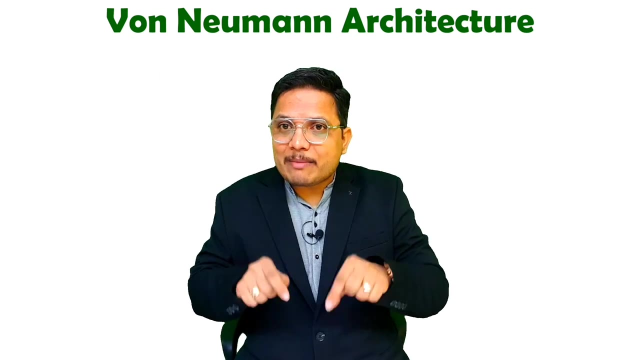 So when it access the data, at that time it may read the data as well as it may write the data. So inside memory we store data as well as program, And as if CPU is accessing memory, which is having data as well as program in the same memory. 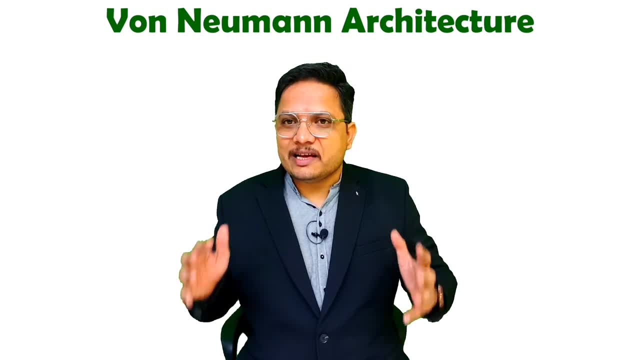 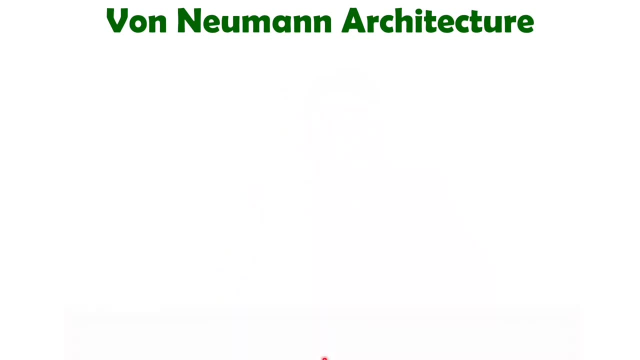 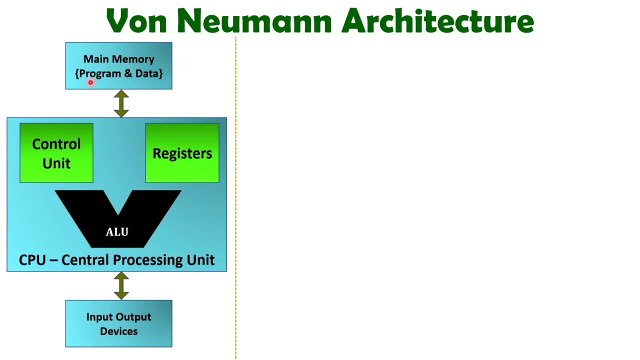 Then you can say this: So this architecture is Von Neumann architecture. Let us see all those things step by step. So here, when we talk about Von Neumann architecture, then you should know, here we have memory, which is having program as well as data. 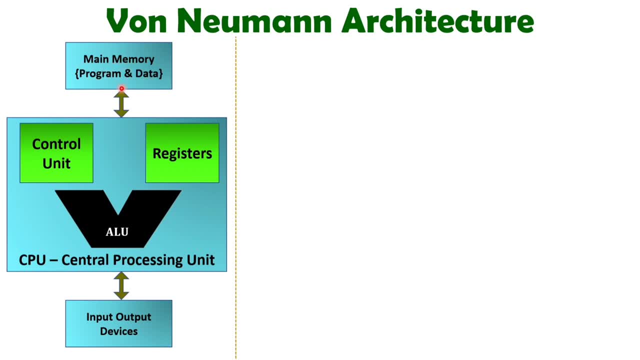 And here, with same memory, we have program and data And by same system bus we access program as well as data with CPU. That's why this architecture is repeatable And that's why it is referred as Von Neumann architecture. So main memory is having program as well as data and that is been accessed by common system bus, right? 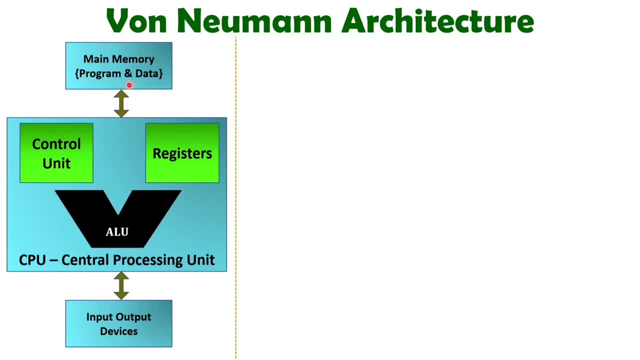 So at the same time you cannot have program execution as well as data access right. Either you have program instruction over here on this system bus or you may have data access right, As we have common buses over here to access this main memory. 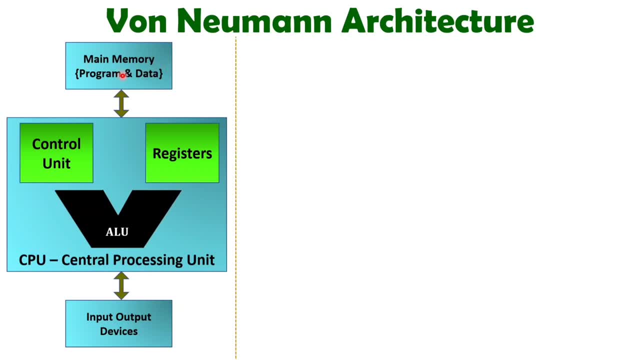 So Von Neumann architecture, That is, having main memory which will be having program and data in the same memory, right? So by giving command by input you can execute any program, right. But at the same time you cannot execute instructions of program and you cannot execute data at the same time along with program, right? 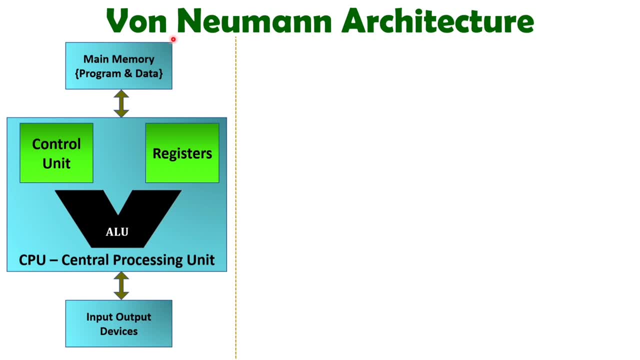 That's why you can say Von Neumann architecture is bit slower Here with CPU, as we know, it is having control unit, Right. So that's why you can say Von Neumann architecture is bit slower Here with CPU, as we know, it is having control unit. 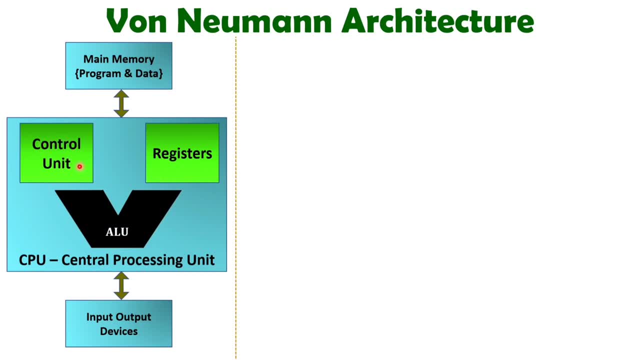 So that's why you can say Von Neumann, architecture is bit slower Here. with CPU, as we know, it is having control unit, Registers and ALU. this control unit is controlling everything. It controls this system bus. it controls internal operation of this CPU, right. 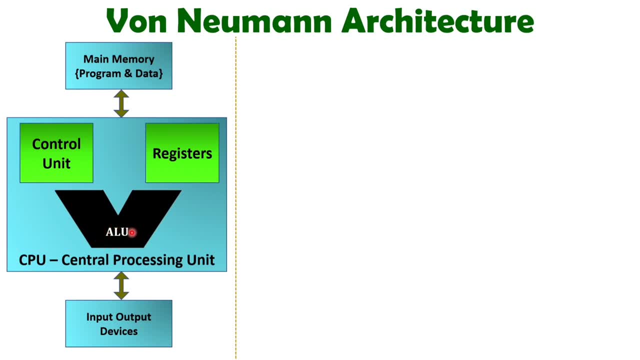 This arithmetic and logic unit that we have it to execute instructions. By input devices, we give command and by output devices we see our output. Let me give you a few more examples, Like when we write any program in higher level language at that time inside program. 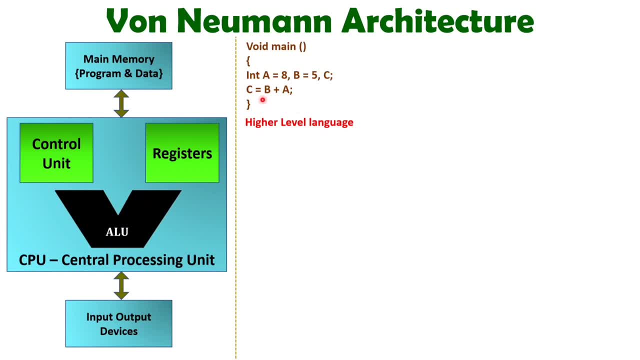 program you will be having instructions as well as data. So you can consider: program executes instructions and data that is also there in main memory, right? So in this same program, you see we have data as well as instruction, Like when you write int: a is equals to 8, b is equals to 5. 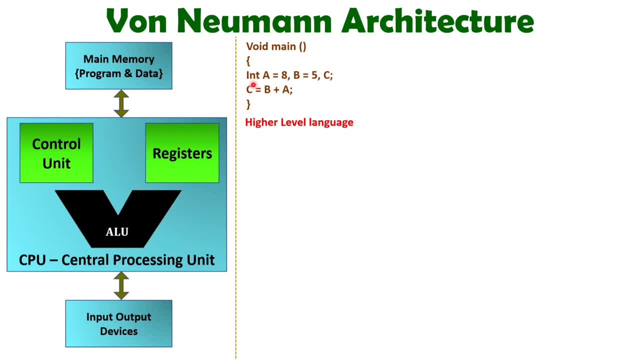 and c. then here you are defining integers where a and b- that is, having fixed values, right- and c is variable, And after that you see what we are writing is: c is equals to b plus a. So this is instruction, which is there based on addition, and these are finite data, right. 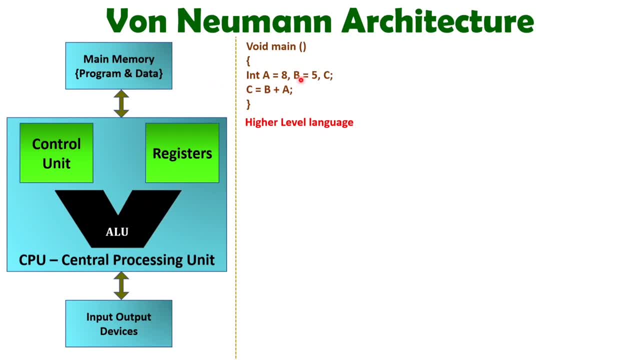 So here with main memory you will be having this data as well as this type of instructions. So when you want to execute any program, at that time you will be executing instructions along with data which is there inside common memory. So when compiler is compiling this program. 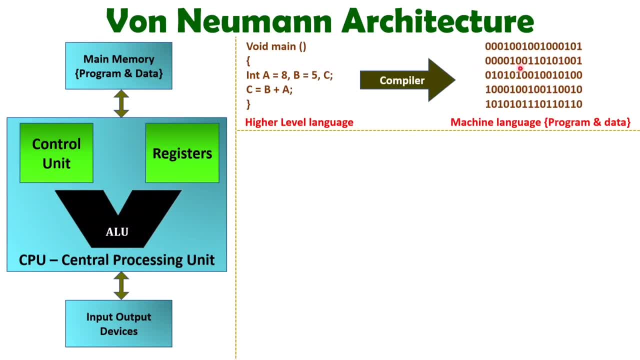 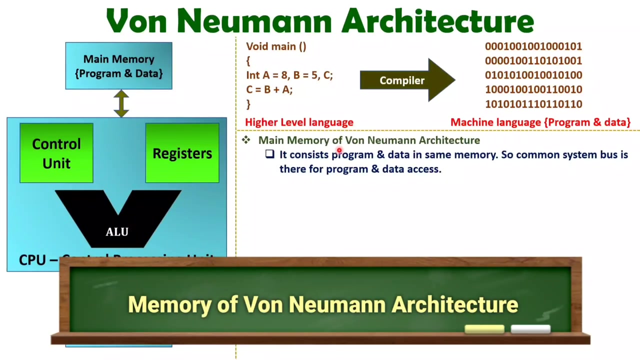 it will be generating binary data, and that is there with program as well as data, right? So program means sets of instructions along with that, data will be there, and program and data, both are stored in a common memory over here With one human architecture. So here, my dear students, when we talk about main memory of one human. 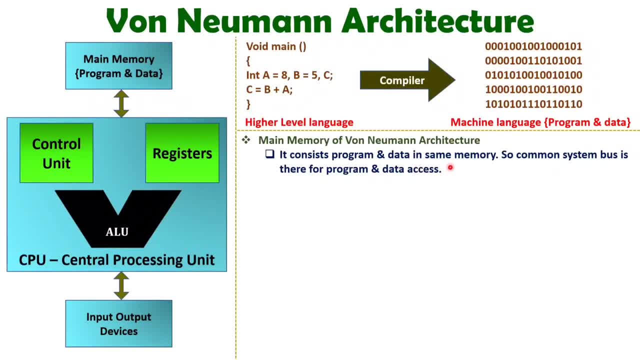 architecture, then it consists program as well as data in a same memory over here, So common system bus that is there for accessing program as well as data Here. when we talk about control unit, then you should know this control unit is providing timing control instruction, fetch instruction. 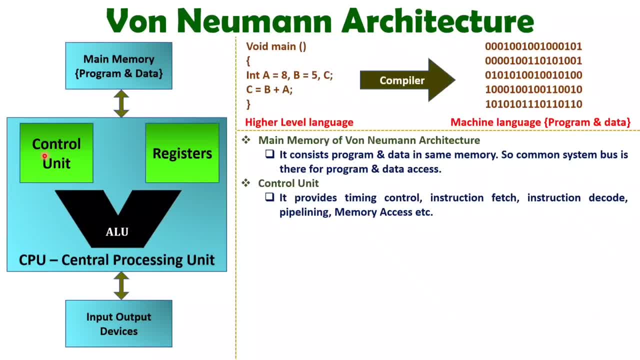 decode, pipelining memory access. Everything is being controlled by this control unit along with CPU. Here, resistors are there to operate with this CPU, So those resistors are having very small amount of memory and that could be operand of this ALU. By using these resistors, ALU performs. 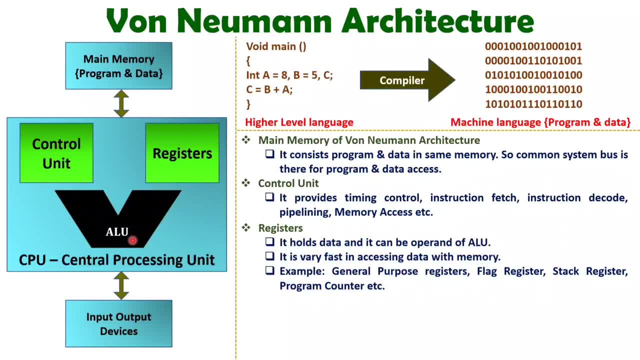 all the arithmetic and logical operations. There can be many resistors inside CPU, like general purpose resistors, flag resistors, stack resistors, program counter. In future coming videos I'll be explaining you general purpose computer along with its resistor organization, so that you can have more clarity about how resistors are there. 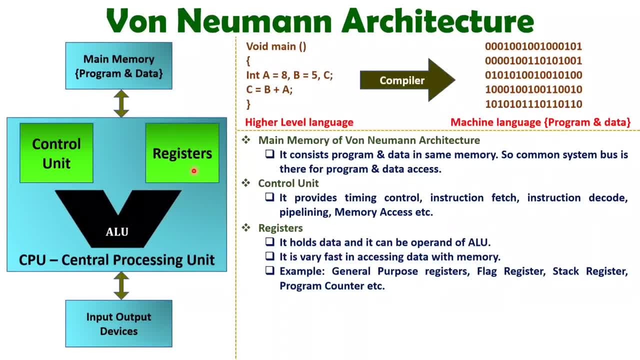 Right now. consider: these resistors are used to execute programs and that could be operand of ALU, and we are executing programs inside CPU with the use of these resistors. only Right here, when we talk about ALU, then it performs all the arithmetic and logical operation like. 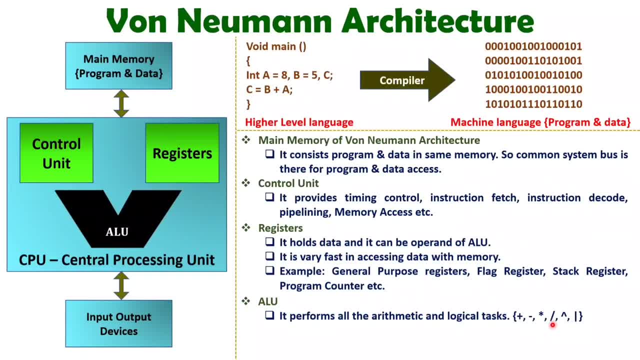 you can perform multiplication, division, addition, subtraction, right, you can perform all the logical operations as well as like AND logic, OR logic, XOR logic, NOT so all those things that is been performed by ALU Here. when we talk about IO devices, then you: 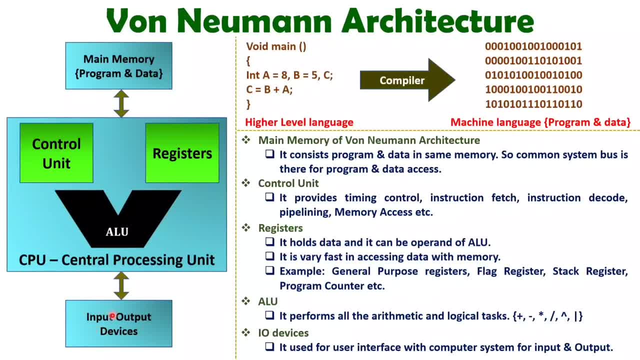 should know to give input commands To input command. we use input devices, like you can have mouse keyboard, as well as output devices are used to see how output is coming. like you can have monitor, you can have printer, you can have speaker right. So, based on your output, you can interface any number of output.